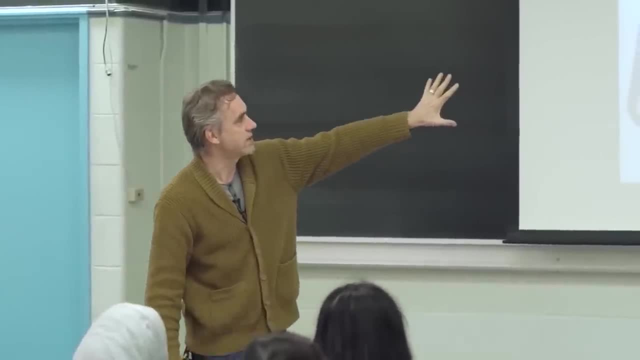 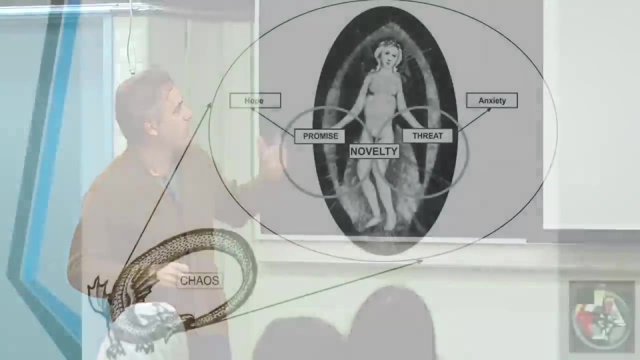 So and so out of chaos emerges this first form. It's the feminine form, It's partly the form that represents novelty as such. So, and on one hand it's promise and on the other hand it's threat that you wouldn't believe and I don't know. 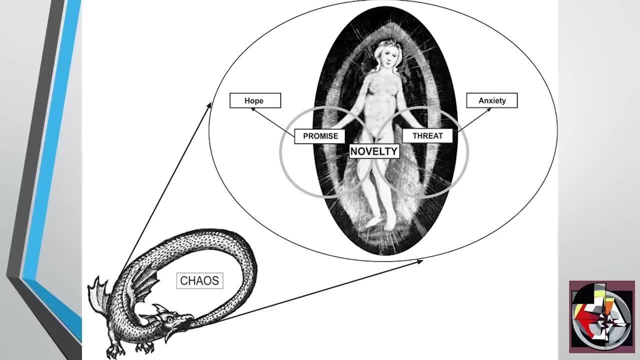 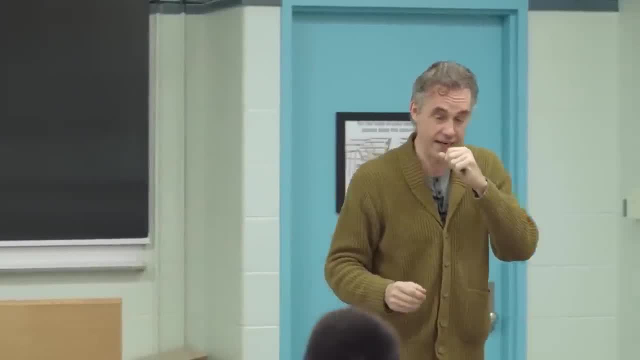 because I don't know. I don't understand the situation with women as well as I understand the situation with men, obviously being a man, But I I don't know if women have any. I don't have any idea how paralyzing they are to especially young men. 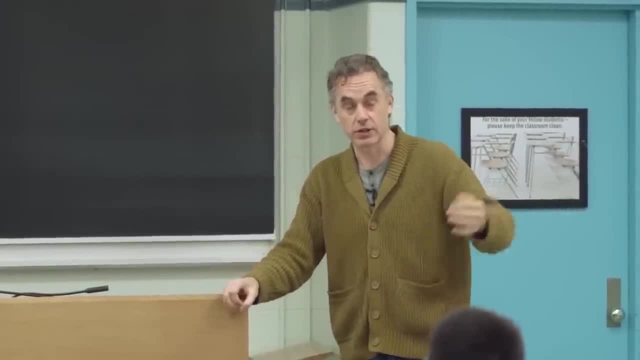 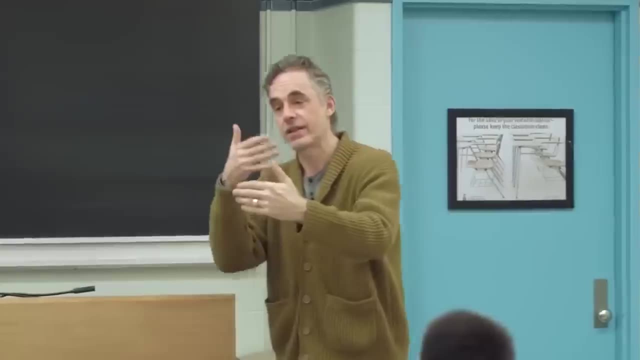 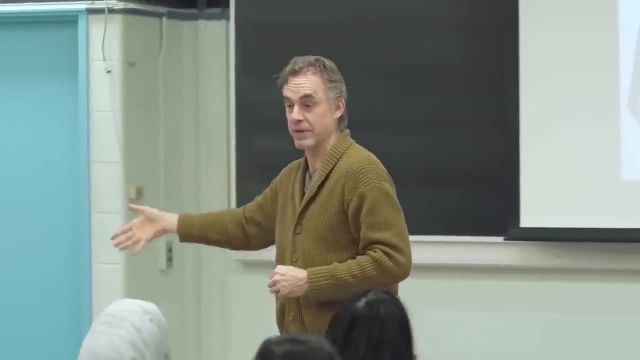 A very large number of my clinical clients, but also young men I've talked to in general, are absolutely terrified of women because they're terrified of being rejected, And the terror exists in precise proportion to the retraction to the woman, which is a horrible, paradoxical situation to be in. 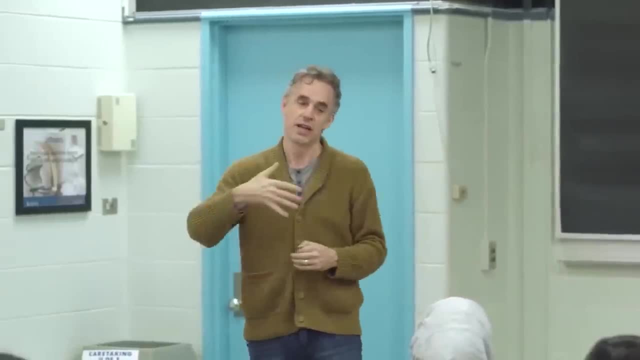 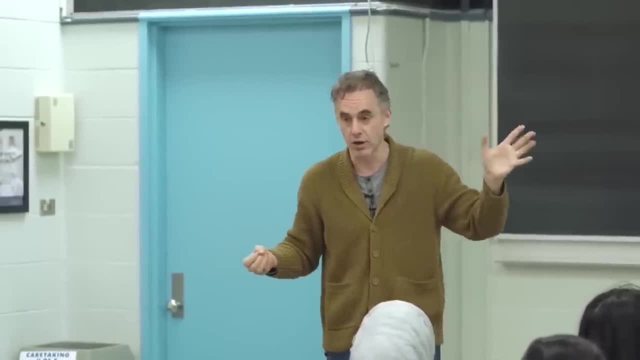 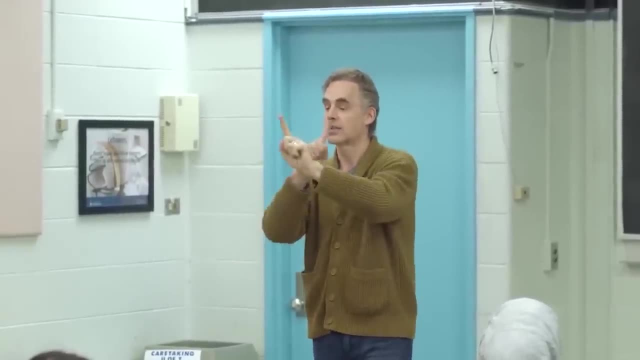 they don't see the woman that they're attracted to because what the hell do they know about her? They don't see her as an individual, They see her as the manifestation of a judgmental ideal. And then it's only in establishing the relationship with the actual woman that they can start differentiating. 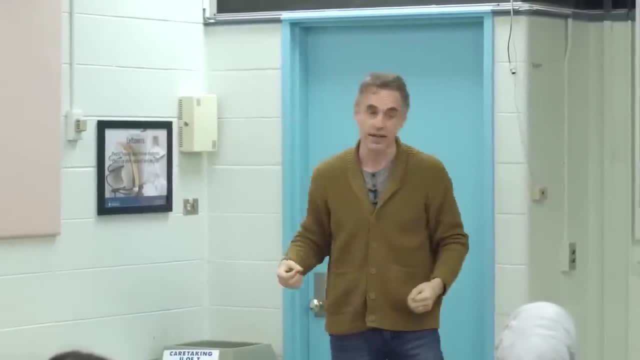 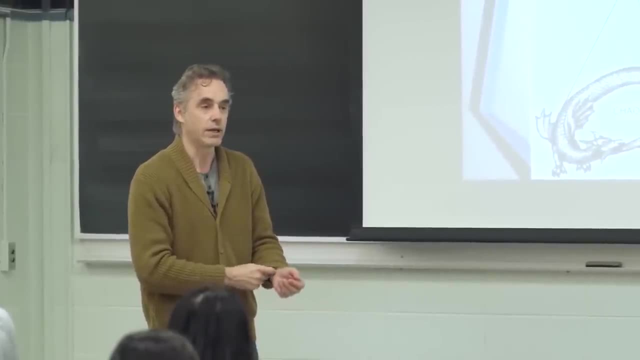 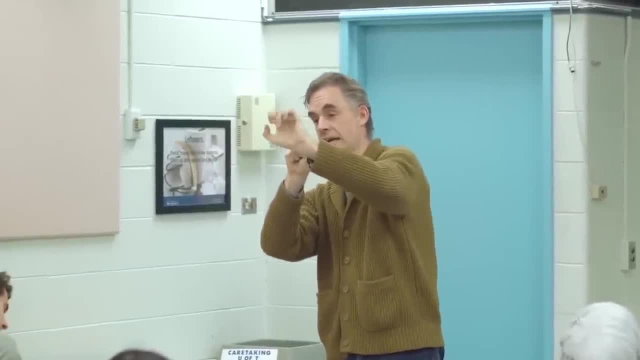 So to have a relationship with any woman, you have to have an ideal woman. So to have a relationship with any woman, you have to have an ideal woman. and sleeping beauty. right, He sees the evil queen, who actually turns into the dragon of chaos.